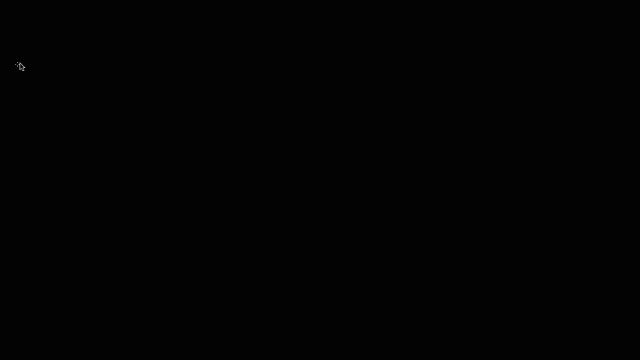 What I'm going to introduce you to in this video is a way to classify numbers as either being even or being odd. So what does it mean to be even? Well, an even number is one where, if you had that many donuts, you could split it evenly between two people. 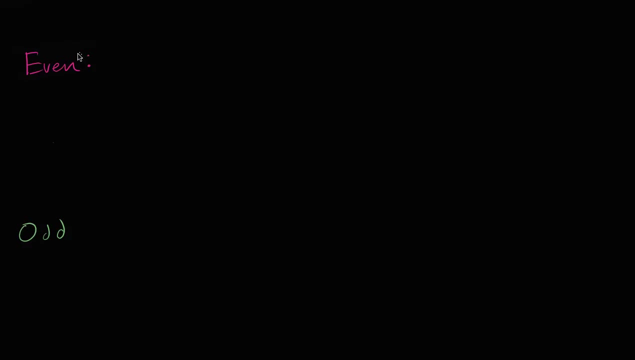 So even numbers are numbers that are multiples of two. So if you have two donuts, you could split them. If you had two people, you could give one donut to each person. Four donuts: you could split that evenly with two people. 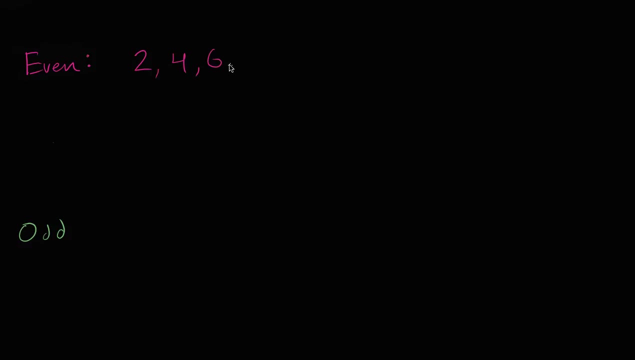 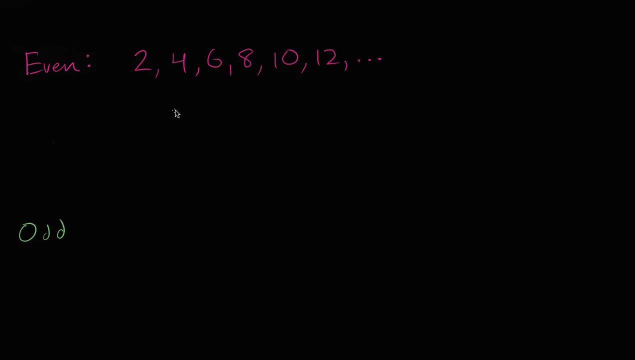 it's ones place is going to be even. So, for example, the number 32 is an even number because in the one's place it's going to be even. In the one's place you have a two, The number 5,977,354,. well, that's an even number. 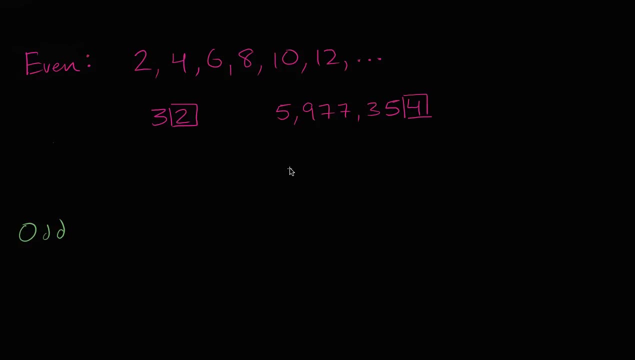 because the one's place is even. Now there's one number, that's an interesting one, why some people sometimes say, well, is this one really even? And that's the number zero. And the number zero is even because it is a multiple of two. 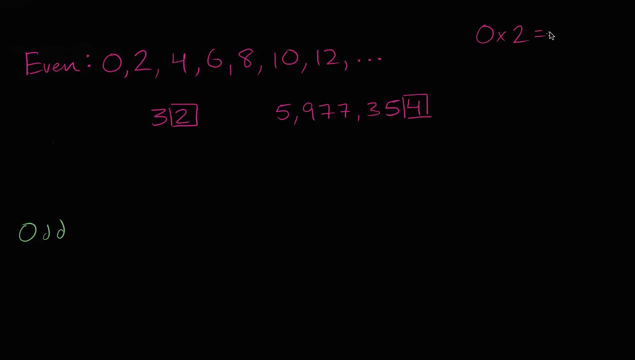 How is it a multiple of two? Well, zero times two is equal to one. Zero times two is equal to zero. So zero is a multiple of two, And so zero for sure is an even number. And then that actually makes our looking at the ones place. 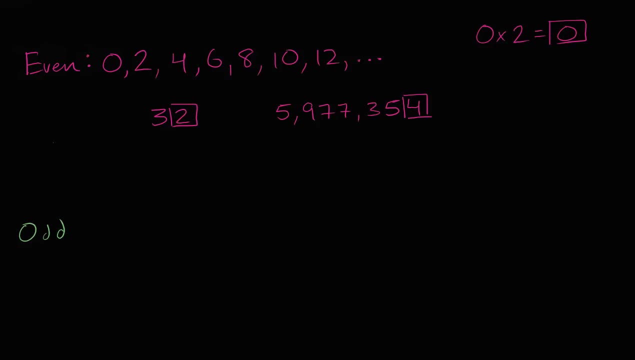 idea hold up, because a number like 150 is an even number And we can look at the ones place of it and say: oh, we have a zero there And a zero is an even number. So if in the ones place you have an even number, 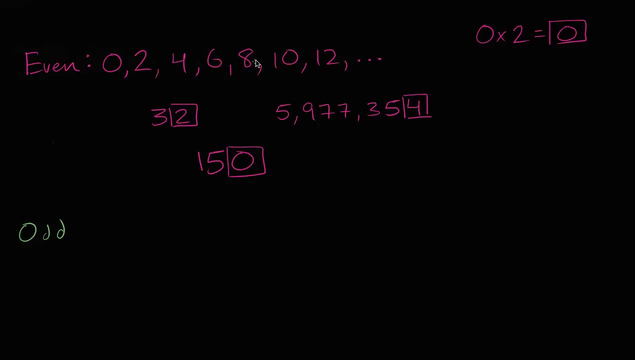 you are looking, the whole thing is going to be even. It's going to be an even number. So what are odd numbers? Well, one way to think about them is they're the numbers that aren't even, So not multiples of two. 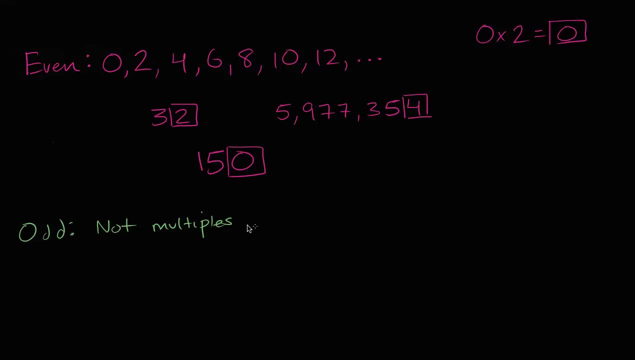 Not multiples of two. So what are some examples of odd numbers? Well, one, three, five, seven, nine, And of course you can go on and on and on. And just like we could look at the ones place to spot an even number, you can also look at the ones. 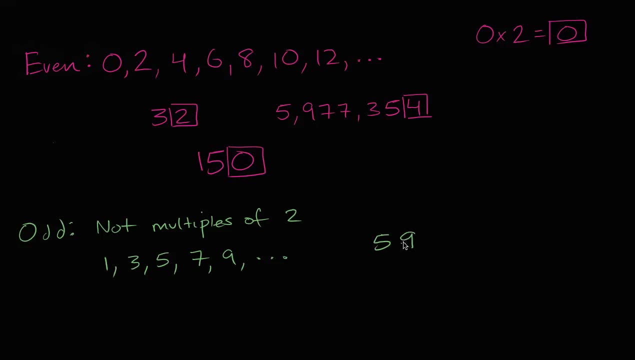 place to spot an odd number, The number 59.. Well, I have a nine over here in the ones place. Nine is odd, So this is going to be an odd number. The number 1,441 has a one in the ones place. 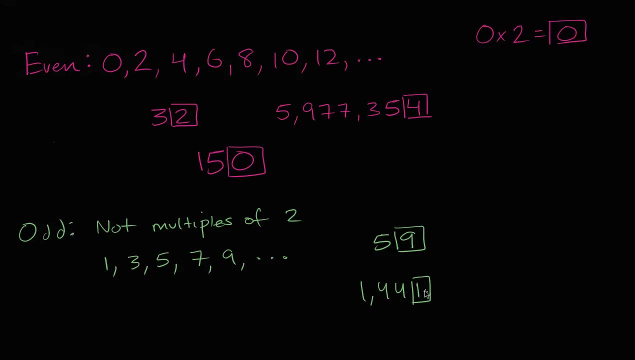 That is an odd number, So this whole thing is going to be odd. And so what's another way of why is it called odd? Well, it'd be hard to split 1,441 donuts. You can't split it evenly between two. 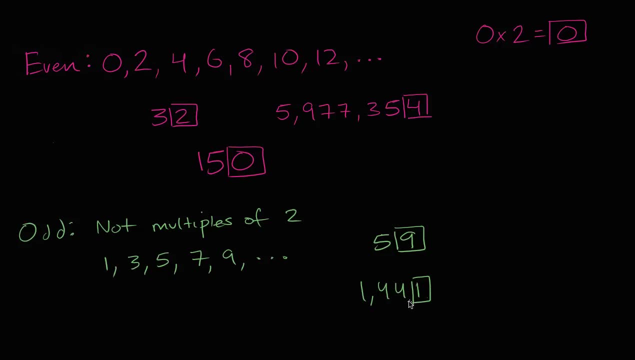 Two people without breaking up a donut. If you wanted to leave the donuts whole, one person would have to get one extra donut than the other person. You can't split it evenly. The easiest way I think about odd, it's not a multiple of two. 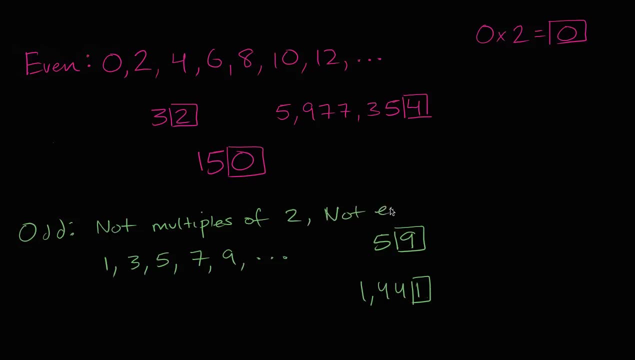 It's not even So. another way, it is not even So. now that we know what an odd or an even number is, let's think about what happens when we operate on odd or even numbers. So let's think in particular. 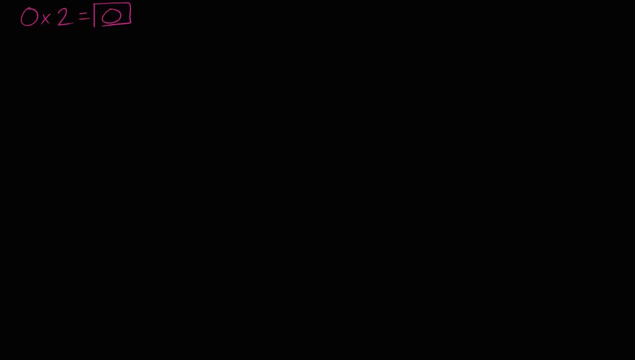 actually, let me move over to the side, right over here. Let me move over right over here. Let's think, whoops, I fell off the screen. Let's think about what happens if I take an even number, an even number plus another even number. 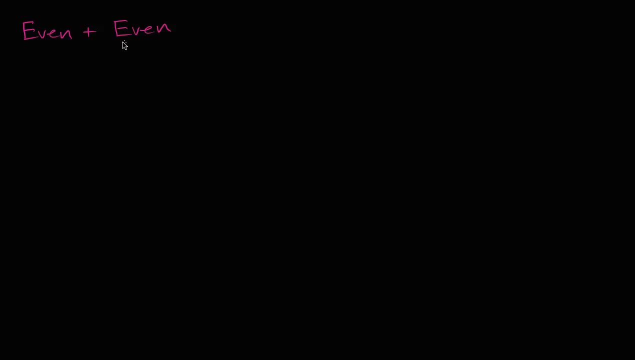 Is this number the sum? is it going to be even or odd? Well, you could take some examples. If I say two plus six, that is going to be equal to eight. Well, eight is an even number. If I say 14 plus four, well, that equals 18.. 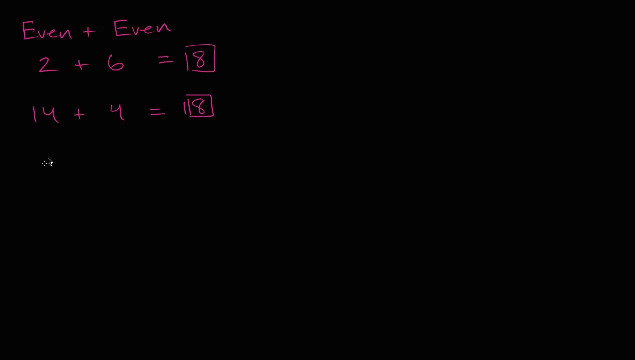 Once again, eight in the ones place. this is an even number. If I say 150, 156, plus plus 100, 100, and let me do a simpler number: plus plus four, that is equal to 160, zero in the ones place. 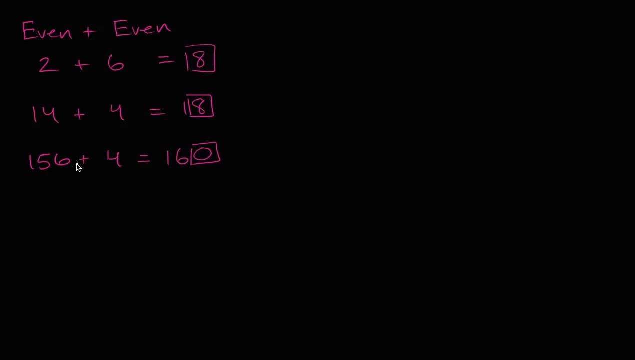 this also is an even number. So it looks like all the examples that I've done so far: when I add an even to an even, I get an even number, And I encourage you to keep trying this out. I encourage you to keep trying. 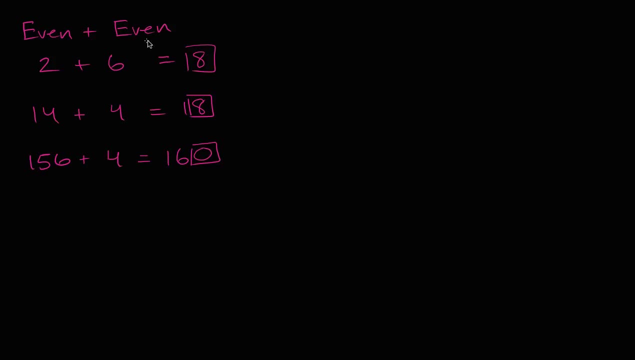 pick some even number, then another even number, add them together and you'll see that you'll keep getting even numbers. And it makes sense, because if you add one number, that's a multiple of two and you add it to another number. 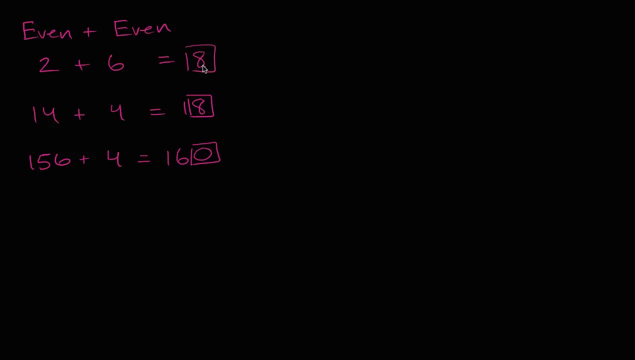 that's a multiple of two. it makes sense, because if you add one number that's a multiple of two. it makes sense that the sum is going to be a multiple of two. Now what happens if you add an odd and an odd? 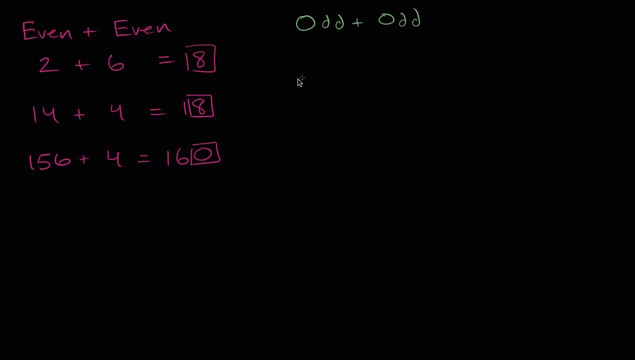 What happens if you add an odd number plus another odd number? Well, let's try. What is one plus three? Well, that's equal to four. You actually get an even number. You add two odd numbers: you get an even number. 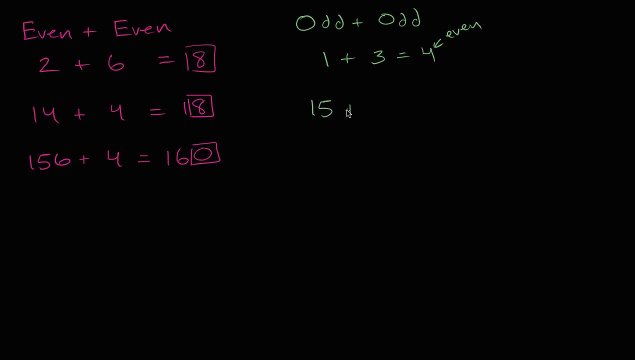 Well, maybe that was just that special case. What if I add 15 plus seven? These are both odd numbers. When I add them together, I get 22.. I get another even number. This is interesting If I take, let me say, 19 plus three. 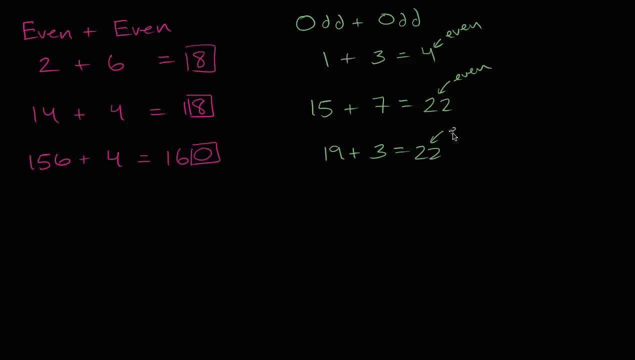 Actually, that gets us to 22. again We have an even number. This is interesting. What about let's see 23 plus five? Well, that gets us to 28. once again, Get an even number. So the pattern that seems to be forming here: 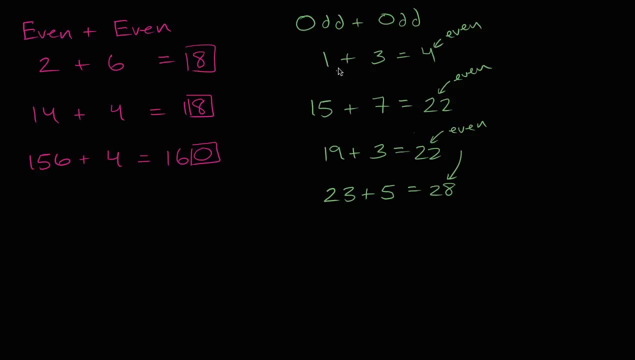 is that if I add an even plus an even, I get an even, but also if I have an odd plus an odd, then I also get an even number. And then, once again, I encourage you to try out as many numbers as you can to see if this pattern holds. 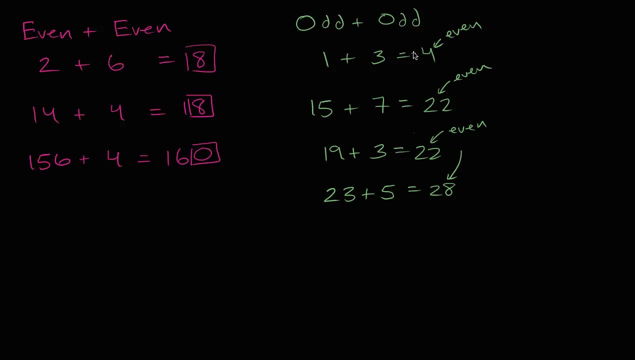 and you will see that it is true. An odd plus an odd number is an even. Now let's think about one last combination. What about an even? what about an even plus an odd? An even plus an odd. So let's say I have two odd numbers. 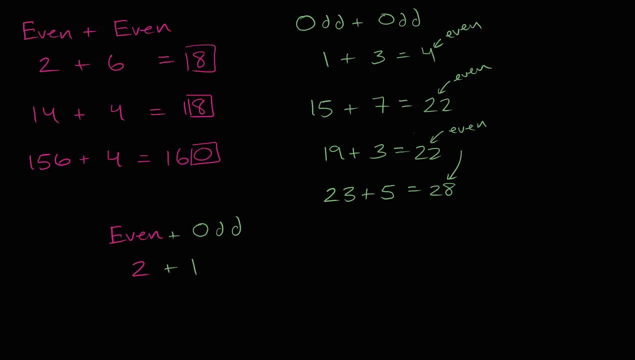 Two plus one. Two plus one, well, what is that going to be? Well, that's going to be equal to three. That's going to be an odd number. Well, what about four plus three? Four plus three? well, that's equal to seven. 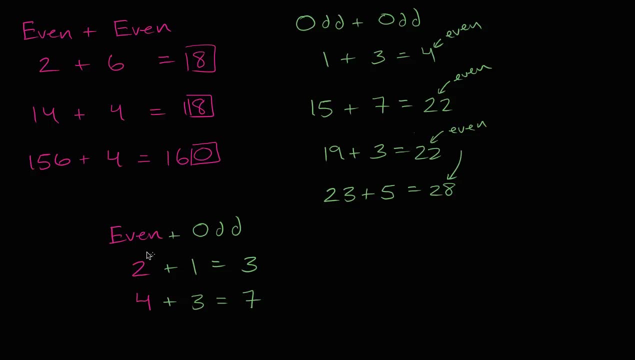 That's equal to an odd number, And so it looks like if I have an even plus an odd- and I've only tried out two cases here, but I encourage you to try out many, many, many more to make sure that you feel good about this. 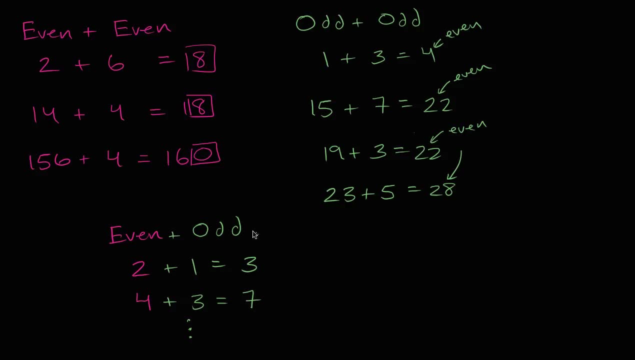 but an even and an odd is always going to give you an odd. So this is always going to give you an odd. So let's just remind ourselves: even numbers, they're multiples of two, including zero. Odd numbers are just numbers that aren't multiples of two. 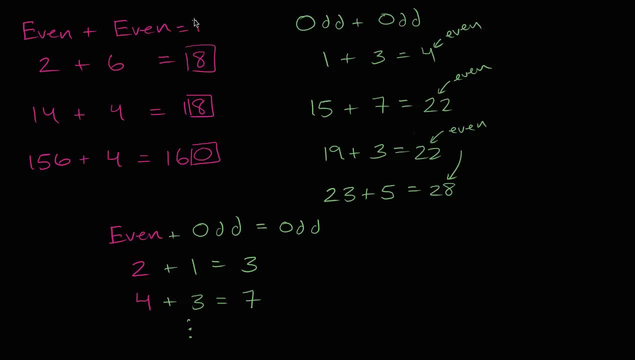 that aren't even, And an even plus an even is going to be equal to an even. An odd plus an odd is also going to be equal to an even. We saw that multiple times. But an even plus an odd, that is odd. And an even plus an even is going to be equal to an even. 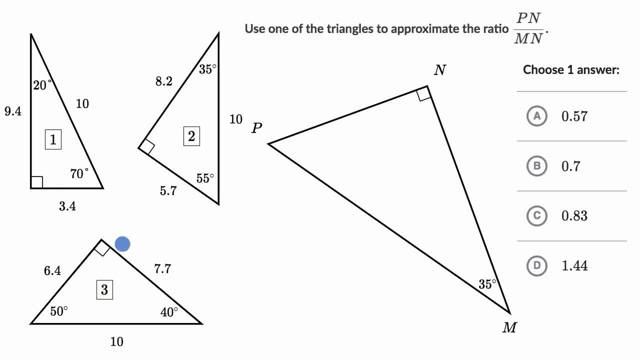 So we've been given some information about these three triangles here, And then they say: use one of the triangles. so use one of these three triangles to approximate the ratio. The ratio is the length of segment PN divided by the length of segment MN. 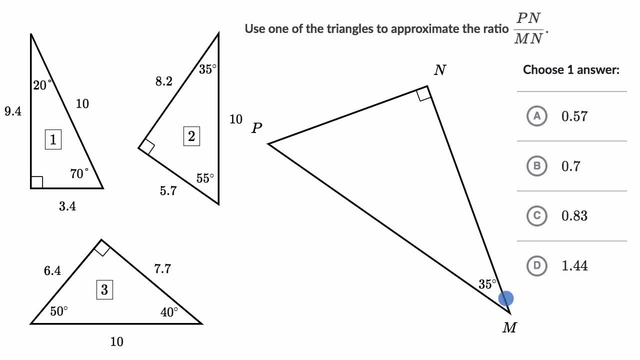 So they want us to figure out the ratio PN over MN. So pause this video and see if you can figure this out. All right now. let's work through this together Now, given that they want us to figure out this ratio and they want us to actually evaluate it. 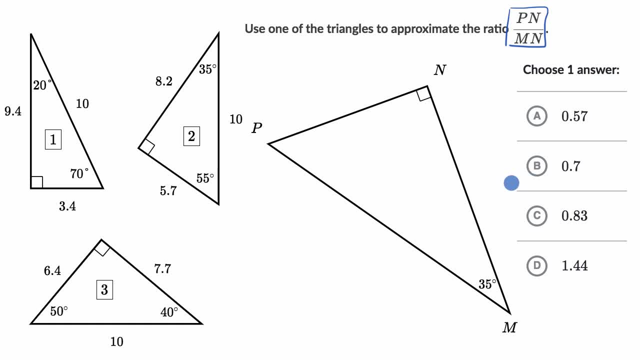 or be able to approximate it. we are probably dealing with similarity, And so what I would wanna look for is: are one of these triangles similar to the triangle we have here? And we're dealing with similar triangles if we have two angles in common. 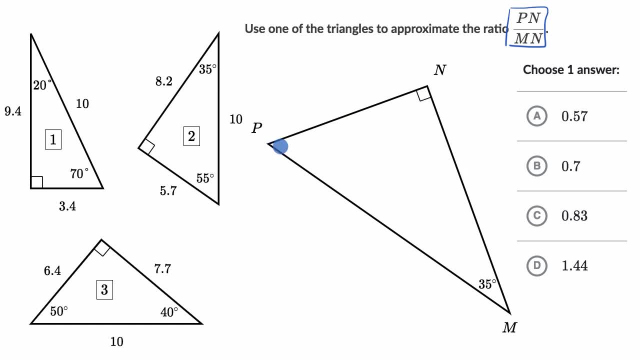 because if we have two angles in common, then that means that we definitely have the third angle as well, because the third angle is completely determined by what the other two angles are. So we have a 35 degree angle here and we have a 90 degree angle here.